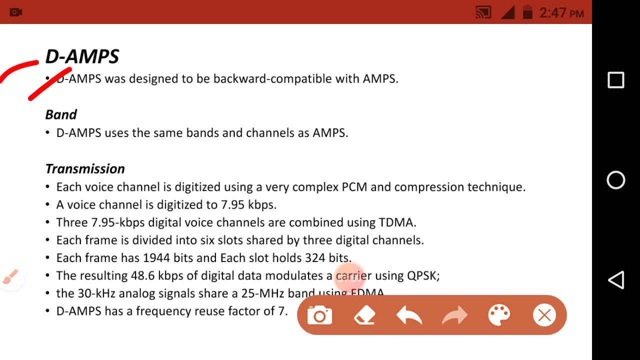 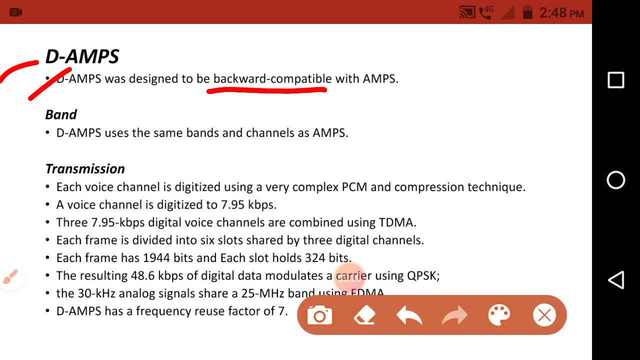 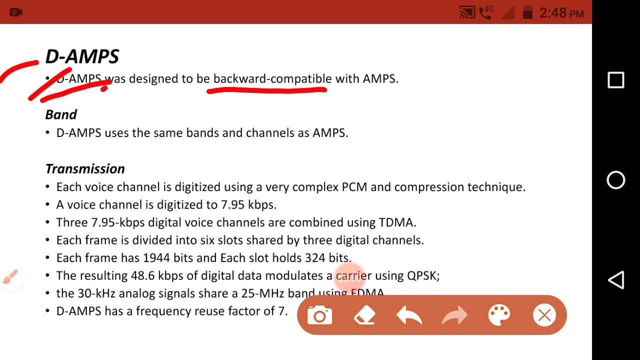 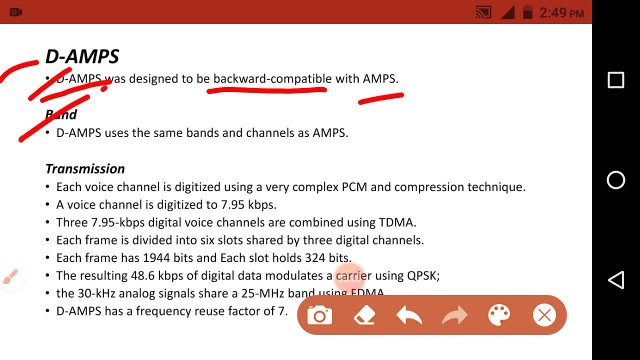 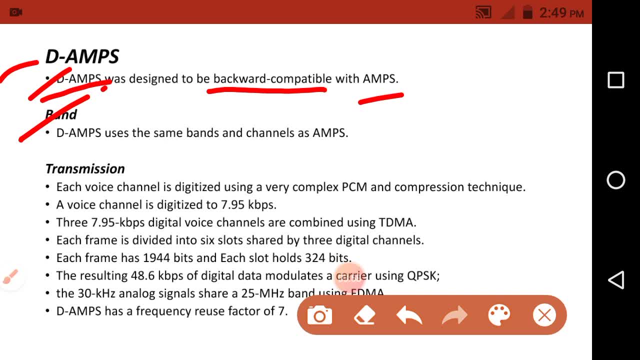 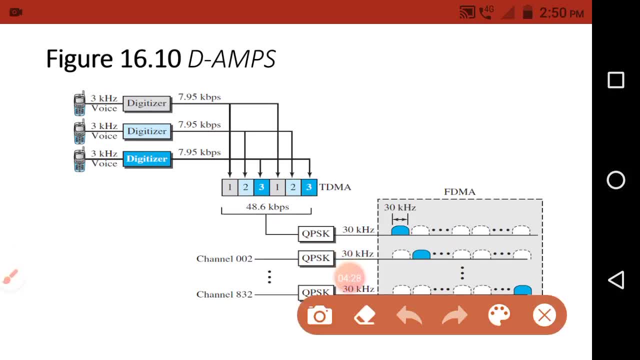 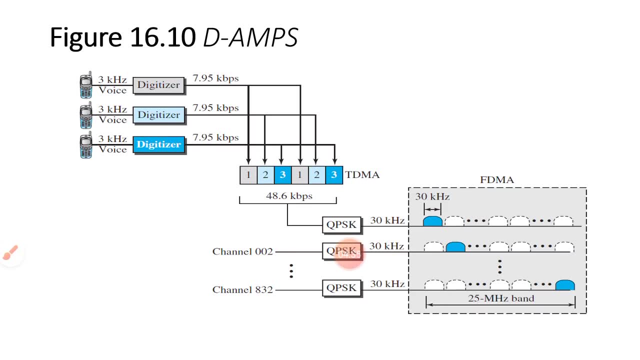 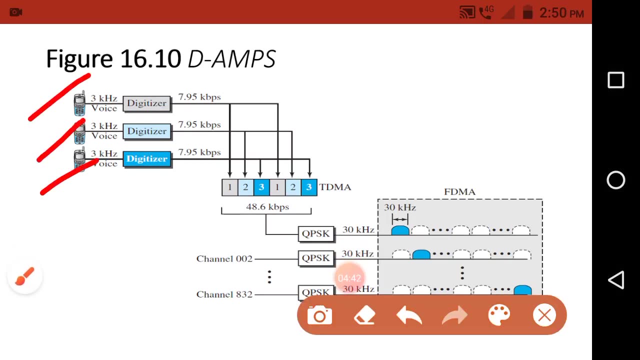 diagram for the digital advanced mobile phoning system. okay, so here. what is the first point? here? there is a. mobiles are there? okay, three mobiles, okay. so each mobile has generated the Y signal. okay, the. the frequency or the bandwidth of that Y signal are three kilohertz. okay, to the bandwidth of the Y signal, this is. 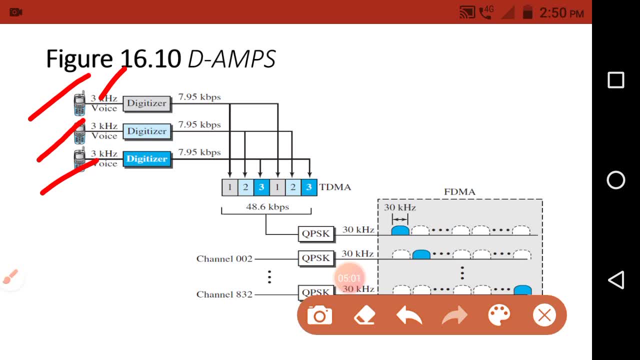 the analog Y signal. okay, and by using the digitizer we need to convert those analog Y signal into the digital Y signal. okay, so that digital Y signal has a data rate we have to call as a data rate in the digital communication of the bandwidth. okay, so that is a seven point nine kilo bit per second. 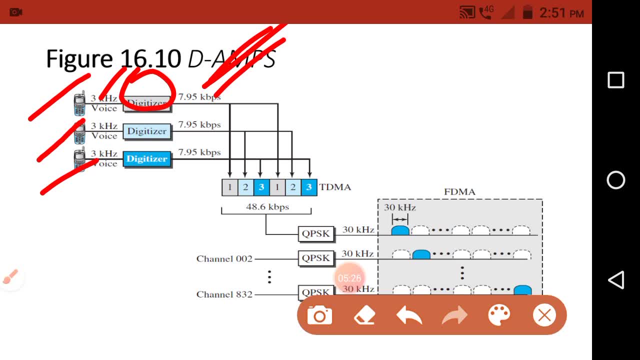 why we have to use the kilo bit per second. so we are representing the digital signal here. that's why we have to use the kilo bit per second to represent the bandwidth of the digital signal. okay, so here, by using the digitizer, we need to convert the analog Y signal of three kilohertz into the 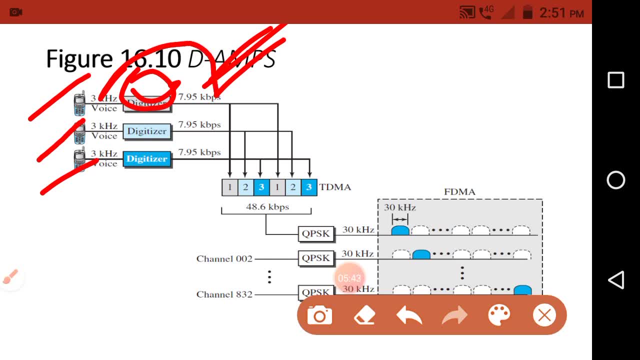 digital Y signal to the seven point nine kilo bit per second. okay, and here we have to use the TDM technique here. so here all these three channels okay, so all these three channels okay, we need to combine here by using the TDM technique. so in the previous module we have discussed the 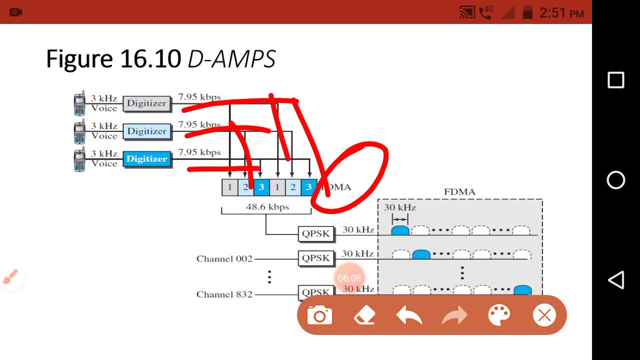 what is the TDM? that is a time division, multiple axis. okay, so here, whole bandwidth of the channel, we can access axis at a given time, although we need to divide the whole bandwidth of the bandwidth of the channel in timely manner. okay, so at a given time one station can access the whole bandwidth of the. 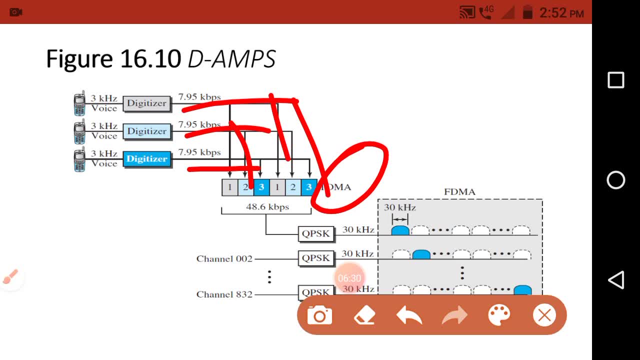 channel and another time the another station can access the whole bandwidth of the channel. okay means in the timely manner we have to divide the whole bandwidth of the channel, okay, so here in this these all three channels are combined by using the TDM technique- time division, multiple axis technique. okay, so 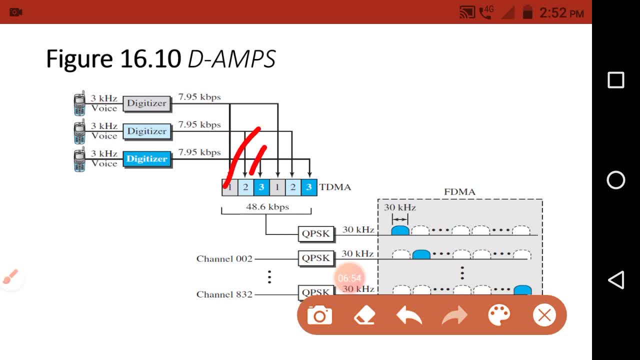 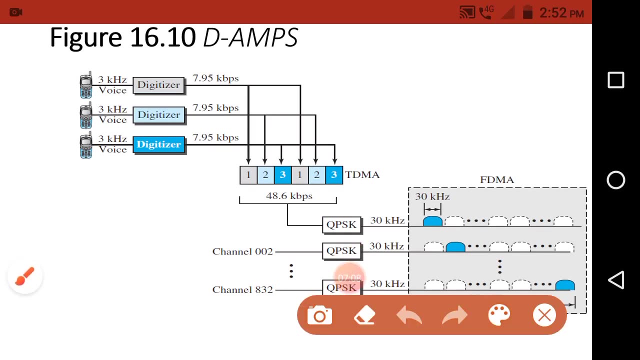 there is a totally six slots are present here. okay, totally six slots. so these six slots are shared among these three channels, okay, and here each channel has get the two slots, okay, so this is the one slot. this is on this. this is a associated with the first. 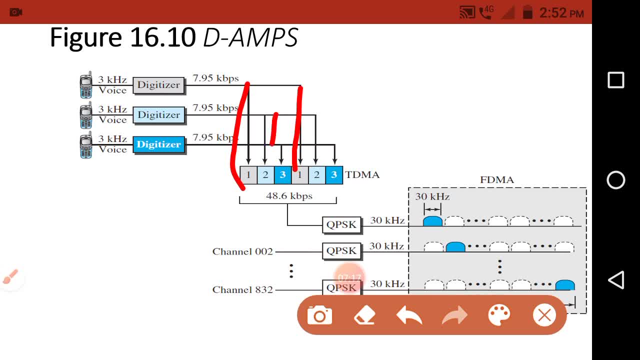 channel okay, and next one is a. this is the second slot, that is, the number second slot- are associated. the second channel- okay, and that is a number three slot has been associated with the third channel. okay means here the e channel has contains the two slot- okay, the channel has contained the two slot here, okay, okay, so there is a. 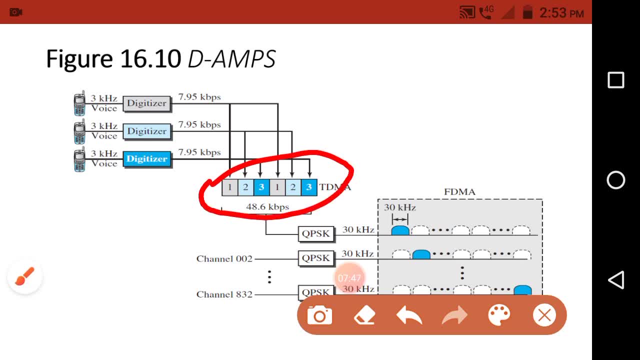 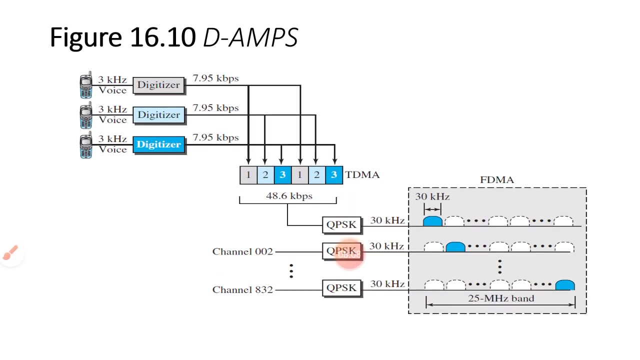 totally, six slots will be formed. okay, so this will we have to call as a one frame. okay, the combination of those six slot we have to call as a frame here. okay, the frame has contains the six slots. those six slots are, say, among the three channels and each channel has got the two slots. okay, next here, so here here. 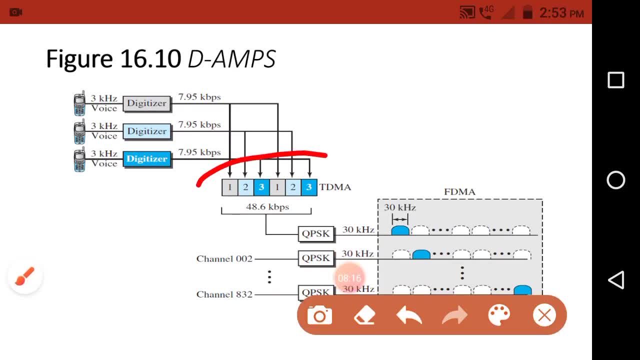 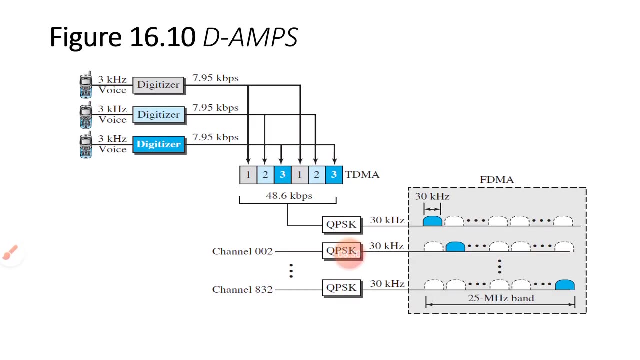 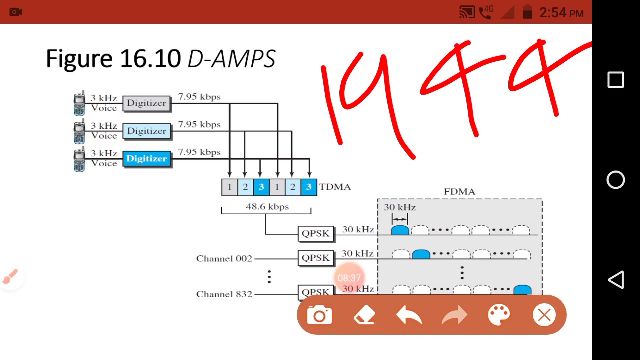 each frame will transmit the. each frame will be transmit nine hundred and forty-four beats- okay, each frame has contains the 944 a beats here. okay, and each slot. so each frame has contains a 944 beats. okay, so this particular frame has contains a six slot. okay, that frame has contains the totally 944 beats. okay, and each slot. 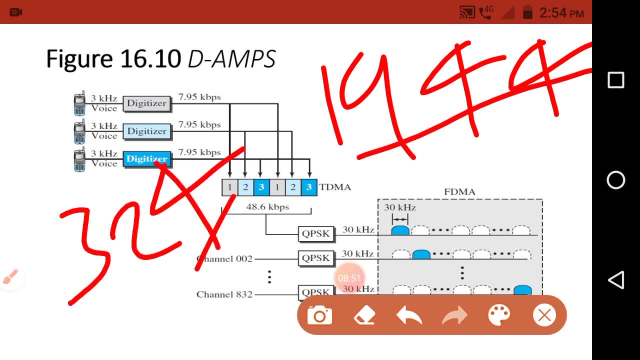 will contains the 324 beats, four beats, okay. so here the sixth slot will will form the one frame. that one frame get one desirable 4-academic has contains a 944 beats, okay, and he slot in that frame has contains the 3, four beats, què, and each slot- there are 5 slots- each in that frame contains the 324 beats, okay, and it will. 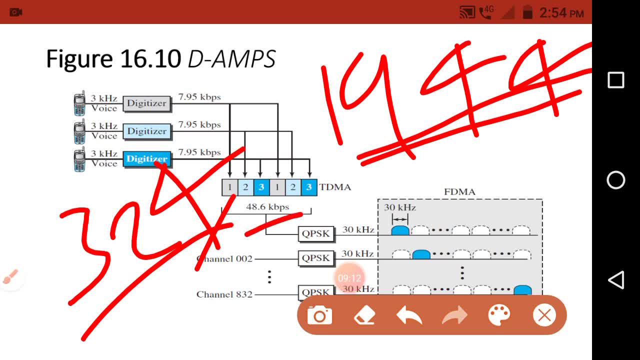 finally result: the forty eight point six ankuy QBR became easy. debate of the. the bandwidth of this is shortweg, four beats матери d the. the bandwidth of the this is four beats merlin g. χ is the p tray of the bandwidth of the. this footرة with zero k Нач 9.6 kTERa. low. it M cyber 13 quitting and it has been present. all this is a head america touch kit played out two nominees, k ciero and it performcell, or sharpening, on which we put out the. we have all the contents of the channel prior to live richard's. that is a. 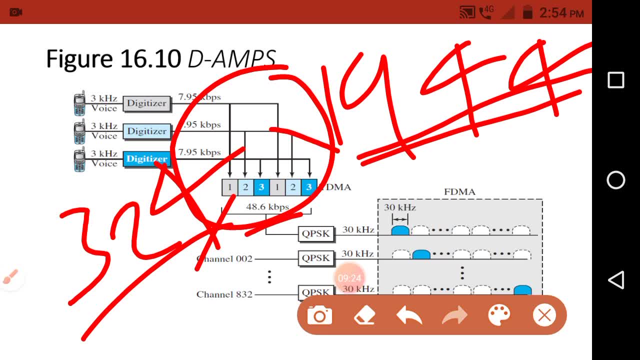 channel. okay, after the combining that over three channels by using the time division multiple axis: okay, so the bandwidth of that whole channel will be forty eight point six kilo beat per second. that is a final beat rate or the bandwidth of the all combined channels. okay, so channels are combined through. 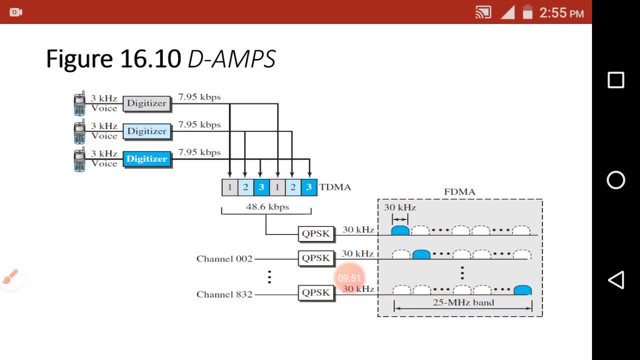 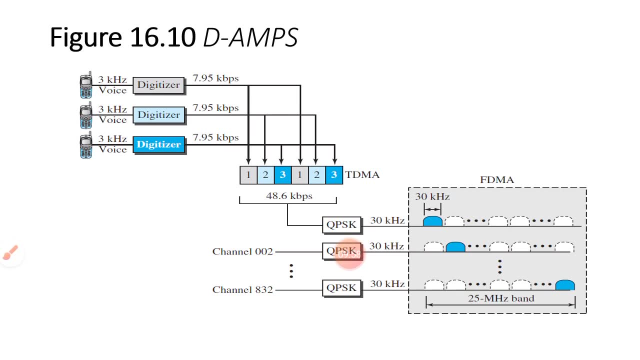 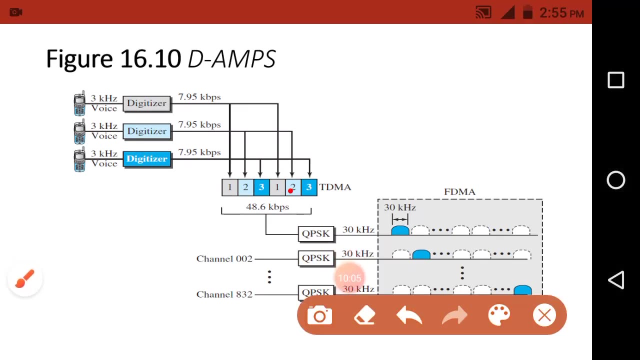 the TDMA technique. okay, so next, this forty eight point six kbps digital signal we need to modulate at forty eight point six. okay, the forty eight point six kbps a digital signal we need to modulate by using the QPSK, that is a. 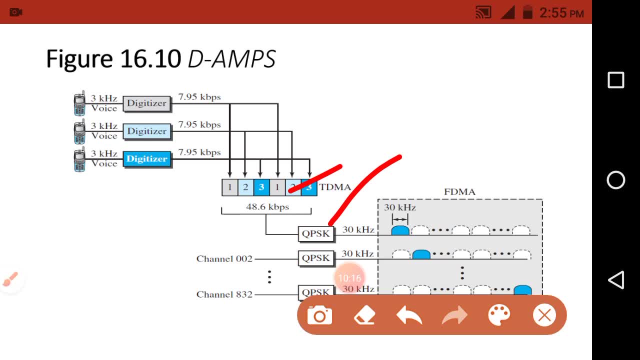 quadrature page shift key already discussed in the previous module. what is the quadrature page shift key here? it is nothing but a combination of two precision king, that is, a two binary page shift key. one is in the in page, another one is out of page. okay, 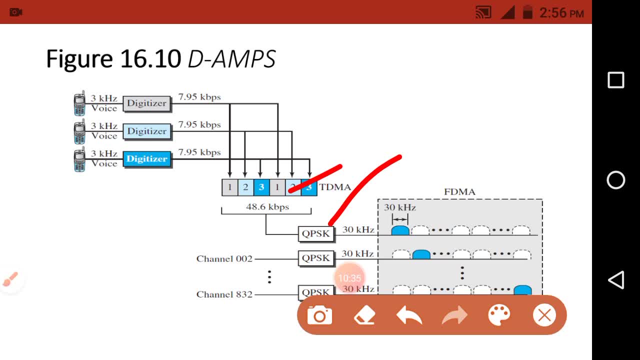 so quadrature page shifting �есп Jessica king is nothing but a combination of two binary page shift key. one binary basic king is in in page and another binary pay shifting king is in out of this. ok, so that's why we have to have to call it is a quadrature phase shift key? okay, so here we need to modulate the digital. 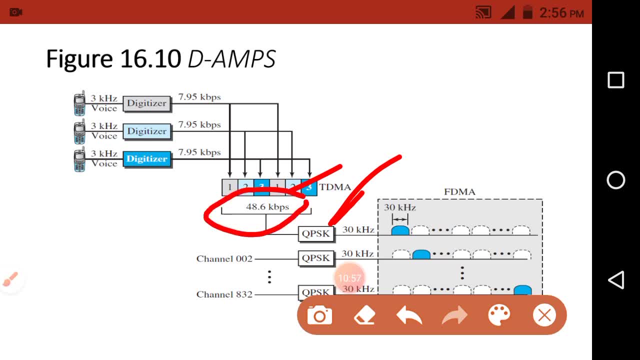 signal of 48.6 kbps into the uh analog signal, that is, a 30 kilohertz analog signal. we already know what purpose we have to use the quadrature phase shift key. the quadrature phase shift king is mainly, we have to use power to convert the digital signal into the analog signal. okay, 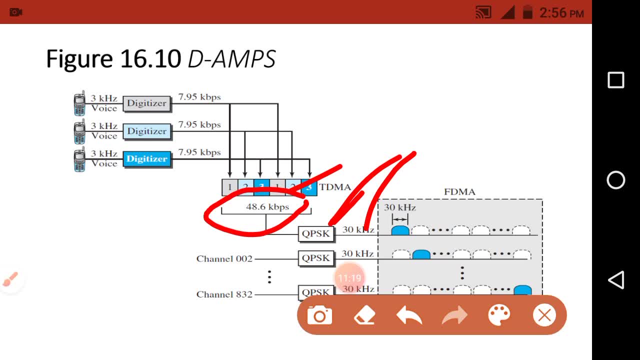 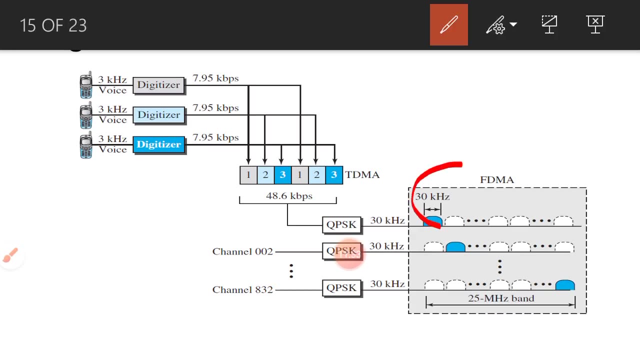 same thing here: the quadrature phase shift king, modulating the digital signal of 48.6 kbps into the analog signal of 30 kilohertz. okay, and after that, here these 30 kilohertz signal. okay, uh, for each 30 kilohertz signal will share the or 25 kilohertz of bandwidth. okay, that is a. 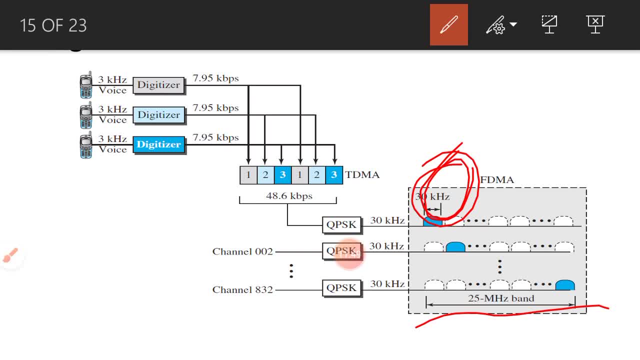 30 kilo signal or the 30 kilohertz channel will share the 25 megahertz bandwidth. okay, so these 25 megahertz bandit, we have to divide it into the 832 channels, as we discussed in the first generation of cellular telephony. so we have divided the 25 megahertz into the 832 channel. 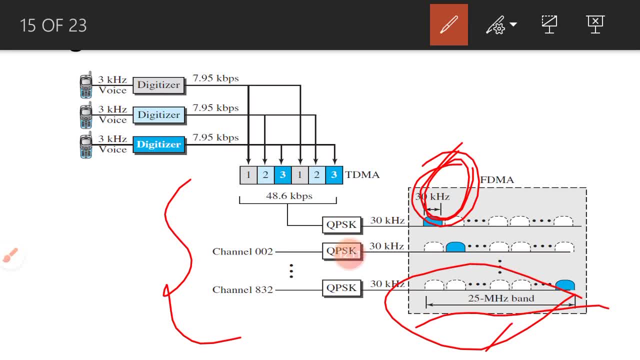 so that is a forward communication as a 32 channel and reverse communication as a 32 channel, and each channel has a 30 kilohertz bandwidth. okay, so here, same thing. this a: we need to divide this 25 megahertz bandwidth into the air 32 channel and each channel has a 30 kilohertz bandwidth. okay, 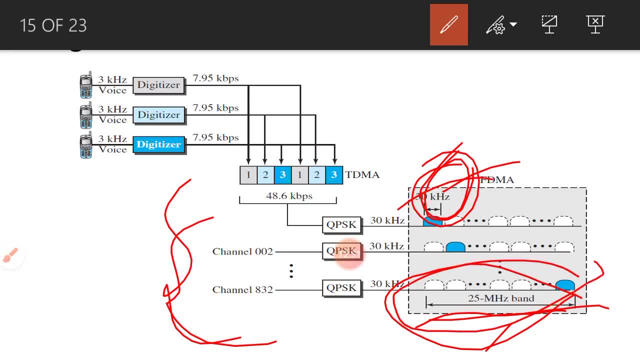 so here this 30 kilohertz bandwidth will share the 25 megahertz bandwidth by using the fdma technique. the prema technique is nothing, but it is a frequency division. a multiple axis okay means here we need to divide the whole bandwidth of the channel. 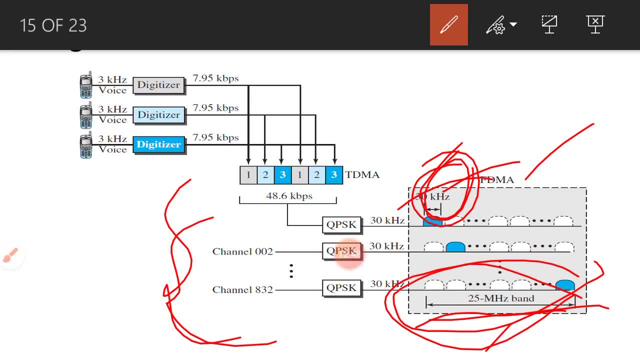 the frequency banks need to divide the whole bandwidth of the channel into the frequency bands, okay, and each frequency band we need to assign to the each station. each station will use that particular frequency band- okay, to access that particular channel or to send a signal to the other devices. okay, so that. 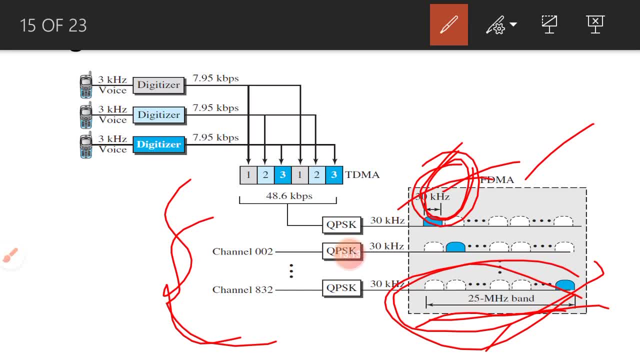 purpose we have to use the frequency division multiple axis. so what is the use of the frequency division multiple axis here? we need to divide the whole bandwidth of the channel into the frequency band and each frequency band is allocated to the station, each station. you will access those banks to transmit. 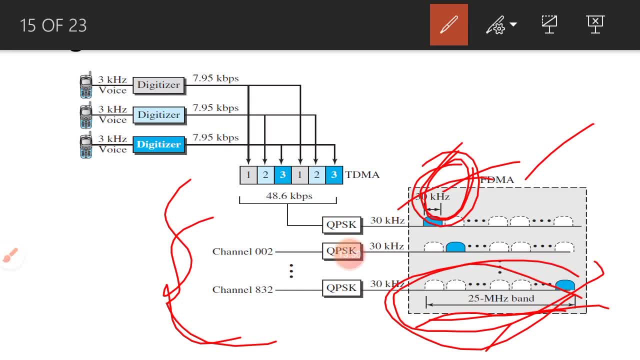 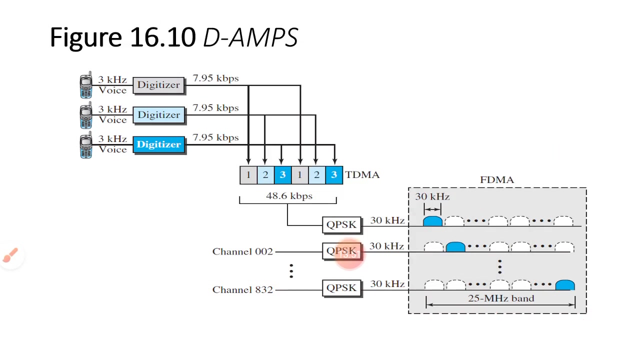 the signals. okay, so that's why here, by using the FDMA technique, we need to divide or we need to share this 25 megahertz bandwidth by using the FDMA technique. so this is a part about the is a. what about the? that is a digital advanced mobile poning system. okay, so. 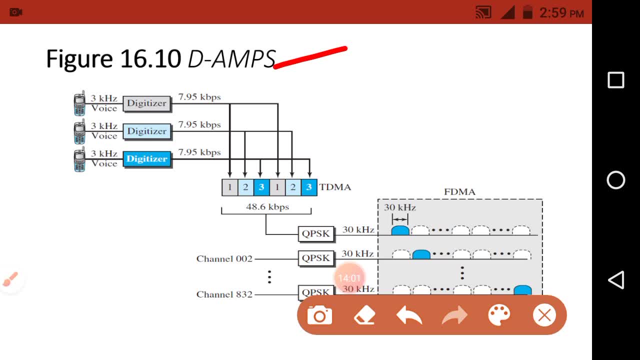 what is our digital advance mobile poning system. so here that first the user will call. that is an analog signal of three kHz that can be converted into the digital by using the digitizer that will give the digital signal of 759 kBps. I Kontor. 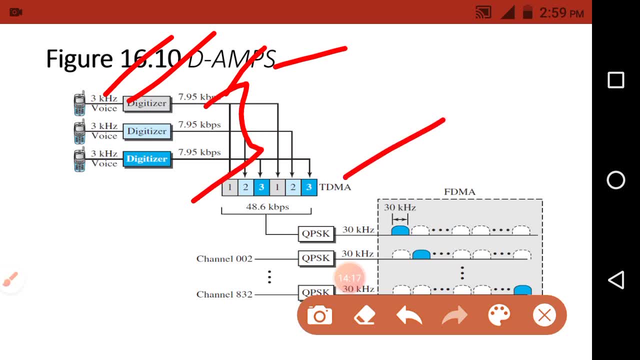 So here, these three signals can be shared by using the time division multiple axis here, Okay, So there is a totally six slots are present, Okay, The six slots are shared among these three channels, Okay, And each channel will get each channel will get the two slots. Okay, And these six slots will form one frame. here, Okay, Each frame contains the six slots here, Okay, And total number of beats present in the one frame, It is a nine frame. 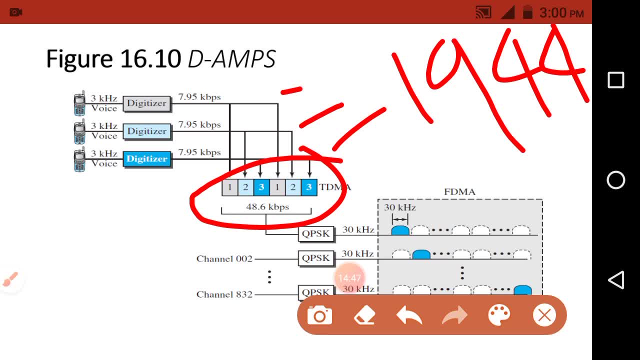 Okay, And number of beats which are present in the frame will be 944 beats. Okay, And number of beats present in the each slot in the frame is that is a 324.. Okay, So 324 is a totally six slot into six. So that will give me 944 beats that will be contained in the frame. Okay, And after that, that will produce the 48 points. 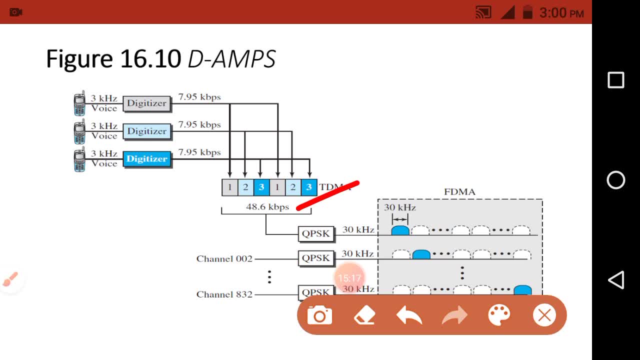 48.6 kilo beat for second. That is a signal bandwidth. Okay, That is a watt output of this particular channel. Okay, That is a 48.6 kilo beat for signal. that can be modulated into the analog signal by using the quadrature pair shift key. Okay, That can be modulated into the 30 kilohertz signal. Okay, So here is 30 kilohertz signal. 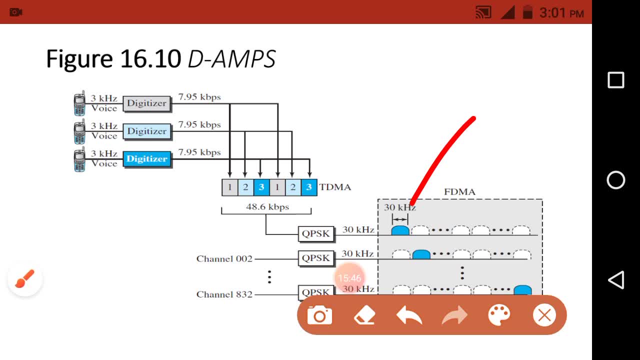 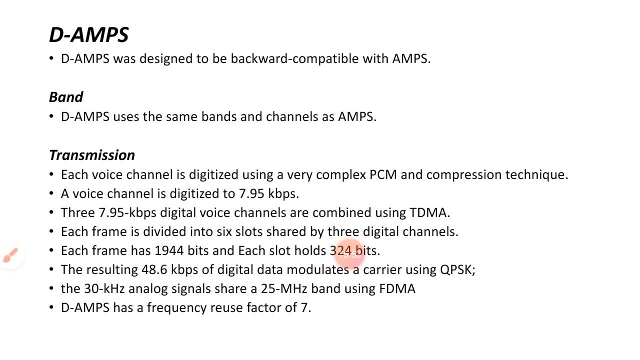 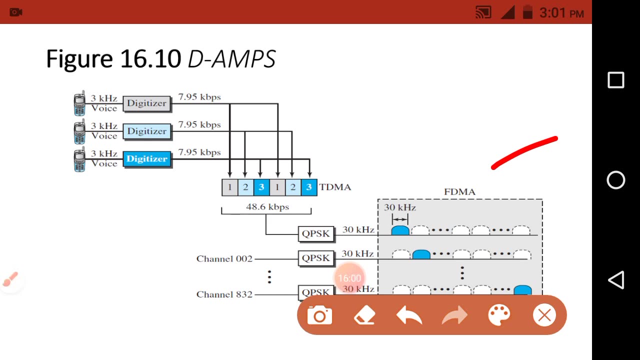 Okay, Each 30 kilohertz signal- Okay, Will share the 20 or 5 megahertz bandwidth by using the FDMA technique here. Okay, By using the FDMA technique, it will share the 25 megahertz bandwidth of the channel And that 25 megahertz bandwidth of the channel, we need to divide it into the 832 channel. Okay, So this is how the communication, how we need to perform the 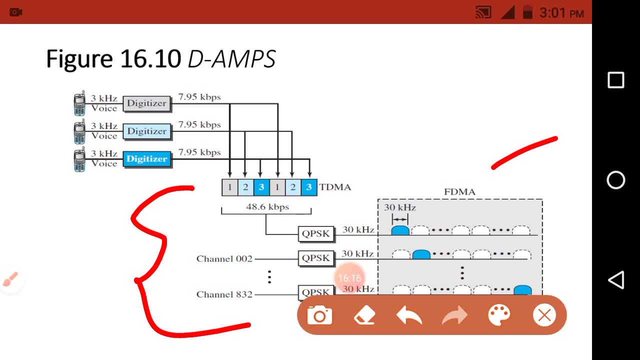 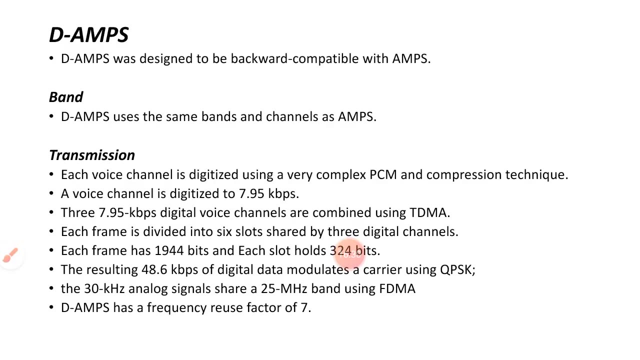 How do we perform the transmission in the digital advanced mobile honing system in the second generation technology? okay, So this is the first one, That is a a Digital advanced mobile system. Okay, So there is another point they argue in the digital Advanced mobile hosting system has the frequency. 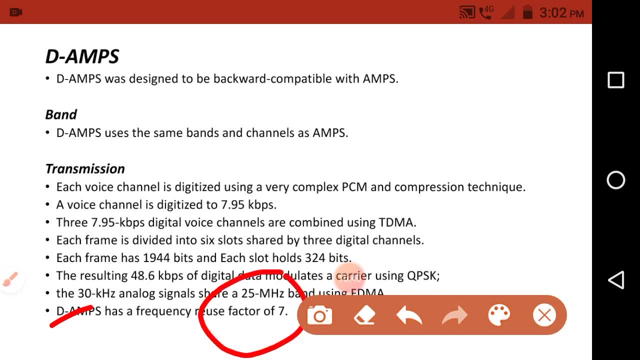 while we need to group the seven cells, how we need to clear the cluster of seven cells here already know what is the reuse factor of a seven in the previous video lectures we have discussed because we need to avoid the reusing: a neighbor cell cannot use the same set. 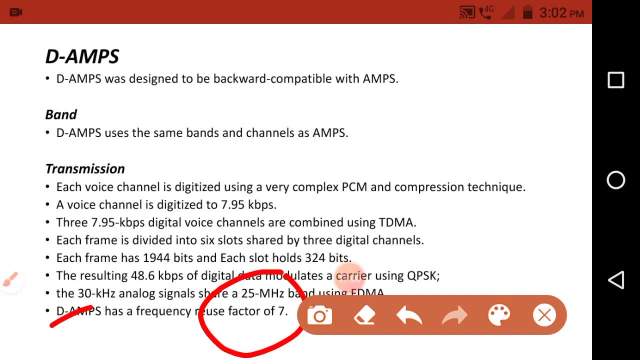 of a frequency. okay, for that we have to use the reuse pattern. okay. so if the same cells are used, the same frequency, that will create the interference disturbance. so that's why you need to avoid the power that we have to use the reuse pattern. so here we have to use them. the reuse factor of 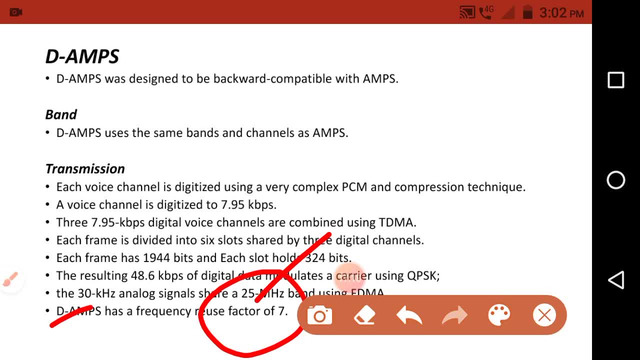 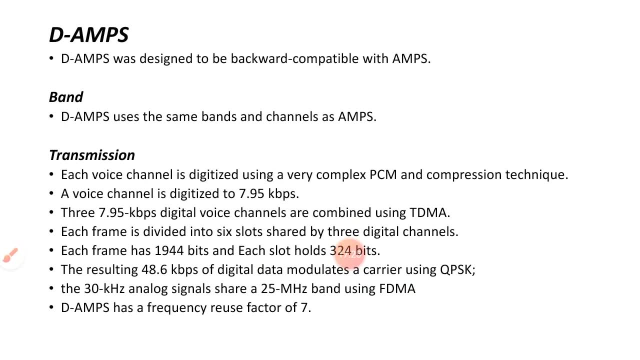 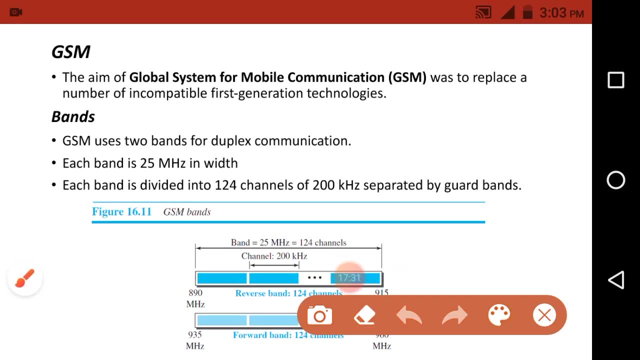 a seven to avoid the interference from the one cell to the other. okay, so this is all about the digital, advanced, digital advanced mobile pony system. okay, and next we will go to the second one. okay, that is a GSM, that is a global system for the mobile communication. 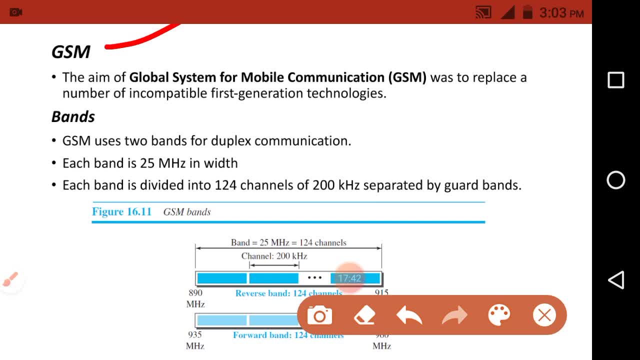 okay, global system for the mobile communication. so is, mainly we have to use to replace the number of incompatibility, okay, number of incompatible, the first-generation technology, okay, that means we need to with this particular global system for the mobile communication we have to use for to. 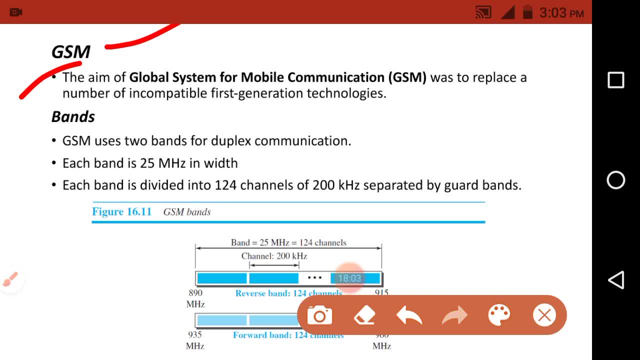 replace the, whatever the difficulty we have to face it at the time of first generation technologies. to replace that, we have to use the global system for the mobile communication. okay, so in that, first we will discuss the bands here. okay, so what are the bandwidth I, what are the frequency range we? 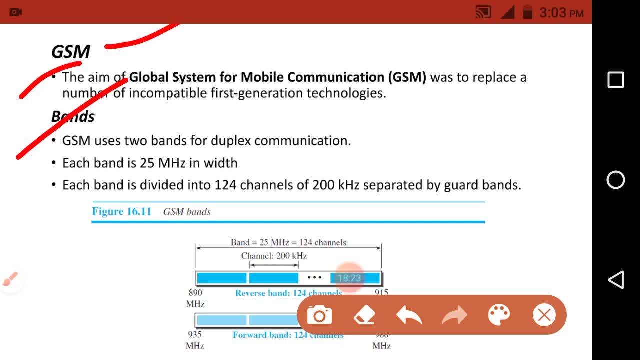 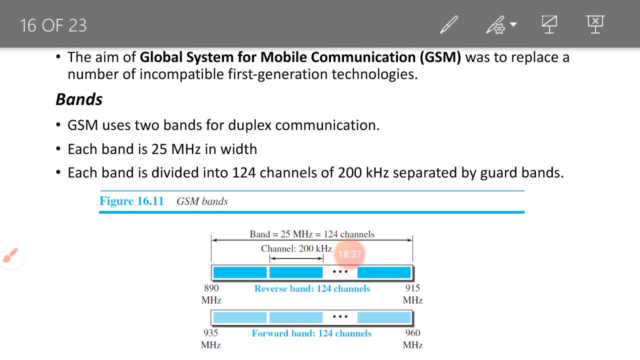 have to use it in this global system, mobile communication. okay, so here. first point: here also we have to use the two bands for the duplex communication. okay, so, as the diagram here indicates, here we have also used the two bands for the duplex communication. okay, two bands means one. 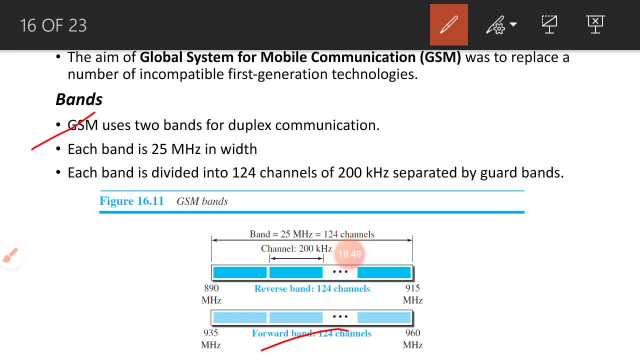 band is a forward band, okay, and another one is a reverse band, okay. so these are the two bands we have to use it in the global system mobile communication. okay, the first one is the forward band. second one is the reverse band- okay. so here the reverse band. 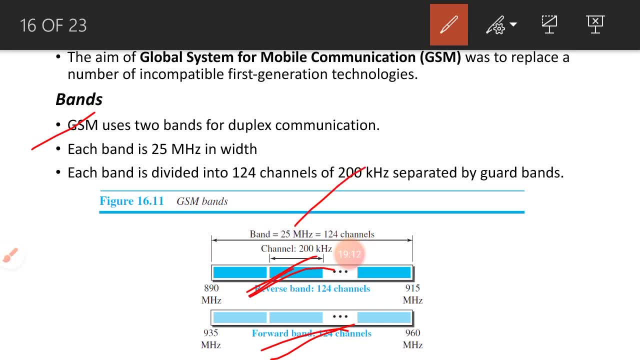 has a 25 megahertz bandwidth, okay, and forward band is also a 25 megahertz bandwidth here, okay. and these 25 megahertz bandwidth, we need to divide it into the 124 channels, okay, and each channel has 200 kilohertz bandwidth, okay. so, and that is a what forward communication and the reverse communication. 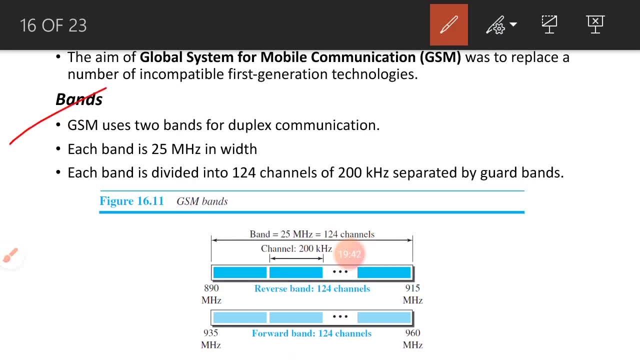 okay, so here there is in the band. there is a. two bands are there? one is the reverse band, second one is the forward band. okay, so the reverse band uh, frequency range is 890 to the 950 and reverse and forward band frequency range will be the 935 to the 960. okay, so means each band has a bandwidth 25. 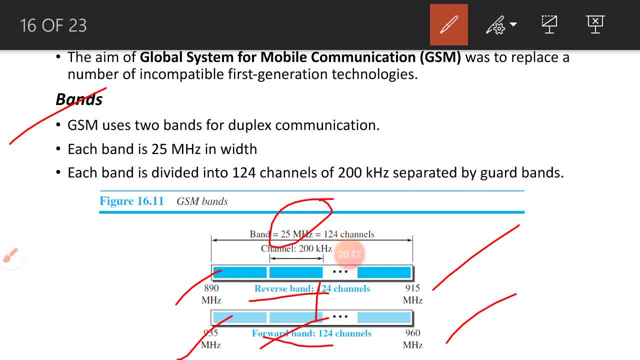 okay, those 25 megahertz bandwidth. we need to divide it into the 124 channels. okay, and each channel has a 200 kilohertz bandwidth. okay, so these are the bands we have to allocated for the global system for mobile communication. okay, so here, forward band and the reverse band, each. 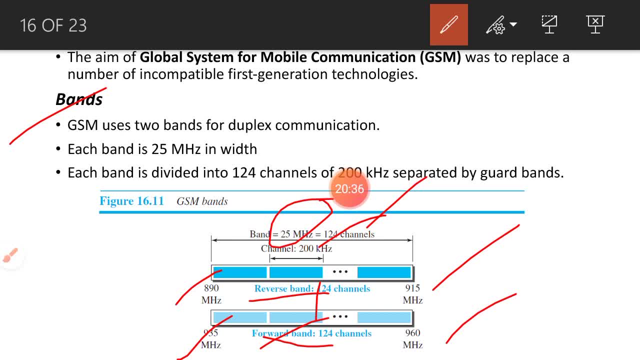 has a 25 megahertz bandwidth and 25 megahertz bandwidth. we have to divide it into the 120 forty four channels, and each channel has 200 kilograms bandwidth. okay, so that is a what bandwidth are you have to allocate it for the global system for mobile communication. 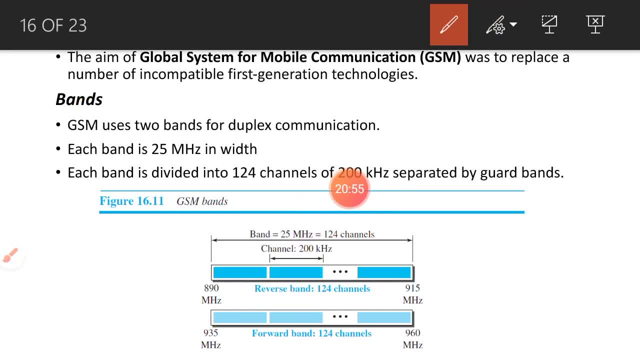 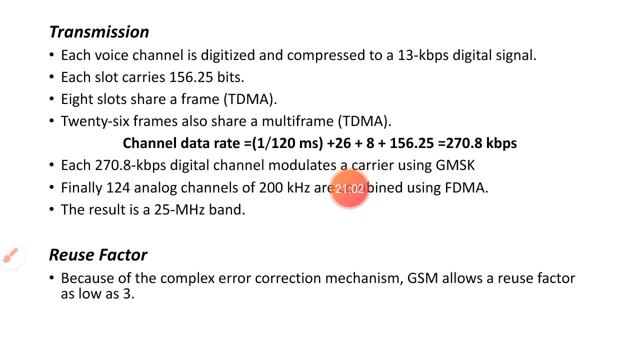 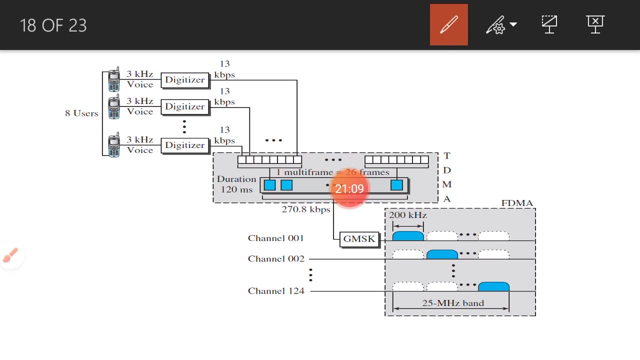 so. so next we will discuss the transmission. so we will discuss the transmission through the diagram here. okay, so here also same thing. the user use the mobile station of the mobile phones to call. okay, so he will transmit the wise analog wise signal, analog wise signal each of three kilohertz, by using 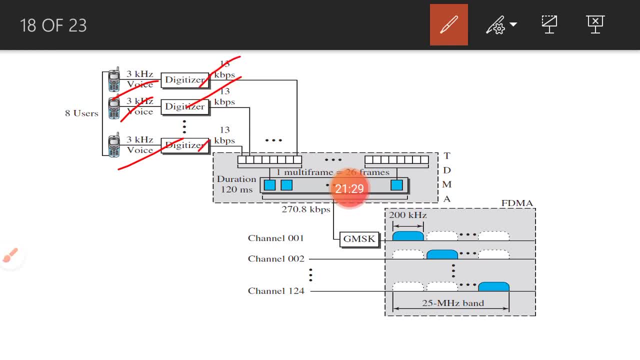 the digitizer, we need to convert those analog wise signal into the digital wise signal. okay, and the bandwidth of each digital y signal is 13 kilo bit per second. okay, and all those channels we need to combine through the tdma technique, that the time division multiple. 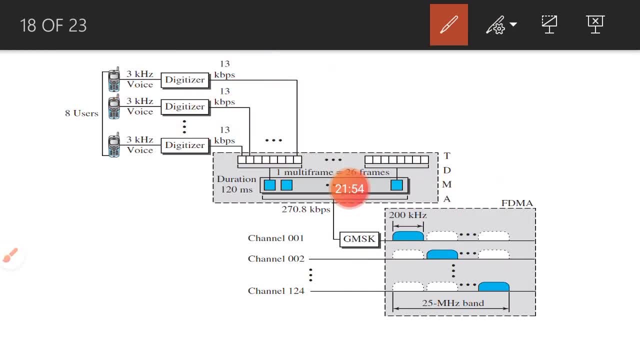 axis. okay. so here here, what happened? the totally eight slots are okay, so the total eight slots are there. all channels are shared, these eight slots, okay, and these eight slots we have to share. the one frame means these combination of these eight slots will form one frame here. okay. 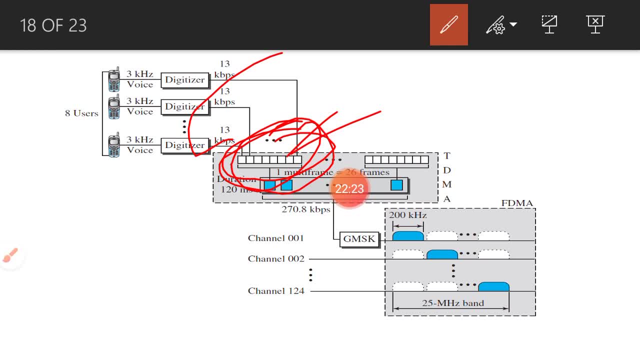 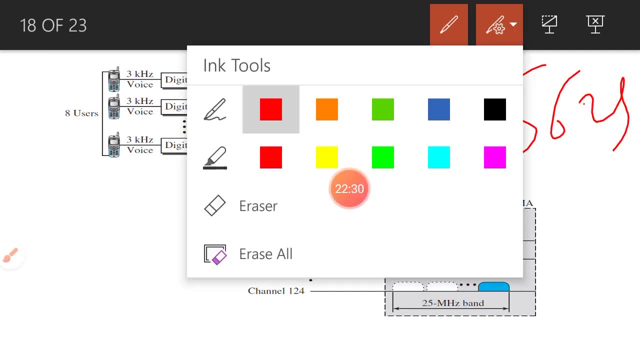 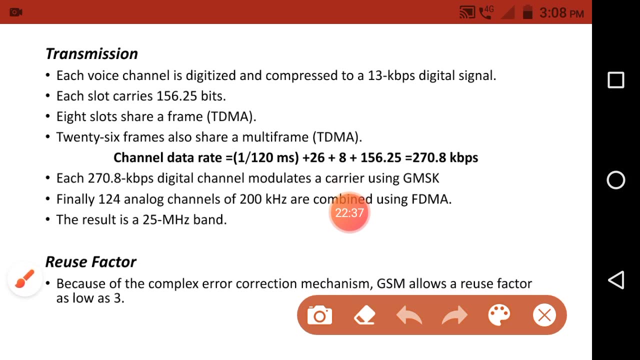 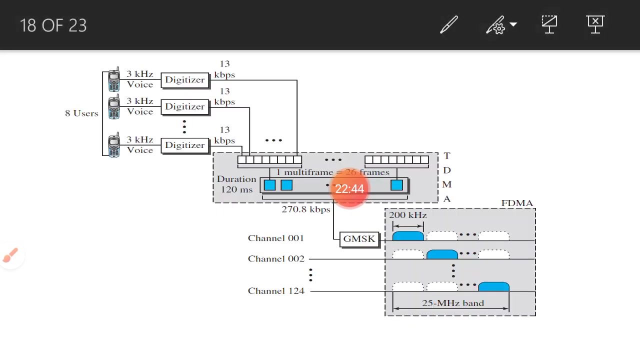 so each slot will contain here 156.25 okay bits. okay, each slots will contain that's what they have given here, okay, so here the each slot will carry one 56.25 beats. okay, so here each slot will carry the 156.25 bits. okay, and these slots will be sharing the each frame, okay, by using the. 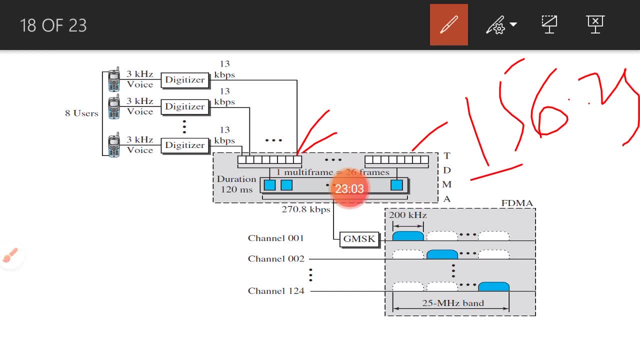 tdma technique, those eight slots will form the one frame. okay, this is a one frame click. okay, that shouldn't be a ten summoner. ok, so let's remember, the one frame set is a recording, okay, and the one frame, okay. so there is a totally. it will send 26 frames here, okay, so through this particular 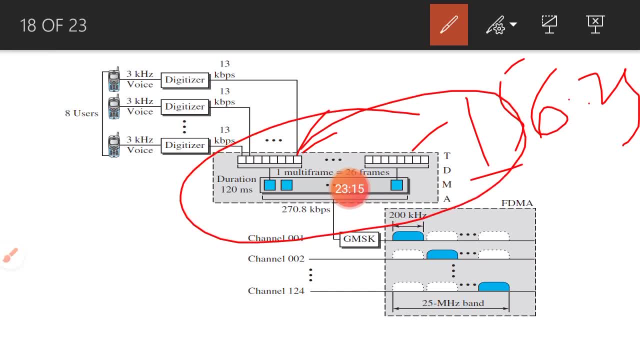 channel, that, whatever the we combine the channel by using the time division multiple axis. so whatever the channel it will form after the combining, so that will send totally 26 frames. okay, so those 26 frame we have to call, as it is a, a multi for multi framework. one multi frame is: 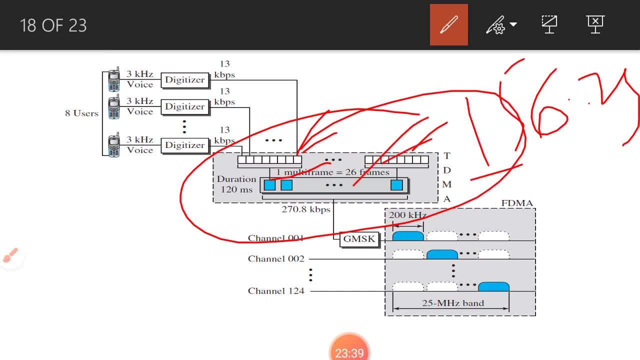 equal to the 26 frames. okay, so those 26 frame we need to transmit to the, this particular combined child, that combined channel, are combined through the time division multiple X's. so here, what is the multi legitimate one multi frame has been to the 26 frame and each frame has contains the eight slots and each slot 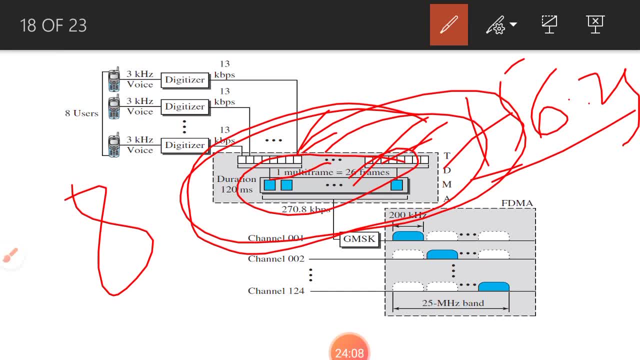 has a 156.25 beats- okay, and these eight slots are shared among the different channels: okay, and after that it will give the total beat rate of the bandwidth of that combined channel will be 270.8 kilo beat per second. okay, and the duration we have to required to send one. 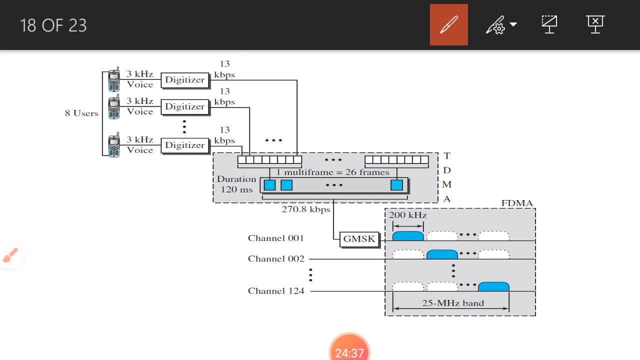 multi-frame is the duration we have to required to send one multi-frame is that is, a 120 millisecond. that 120 millisecond we have to required to send one multi-frame, or the 26 frame through the channel, with the channel bandwidth has been 270.8 kilo beat per second. 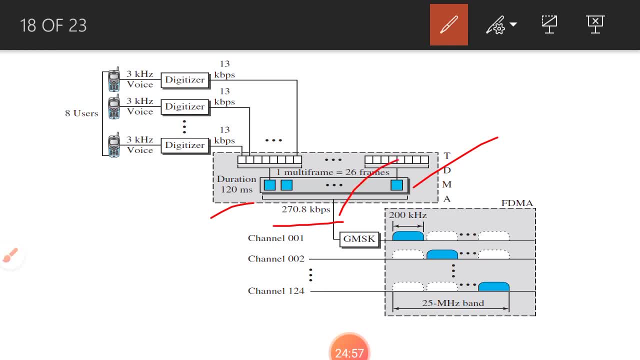 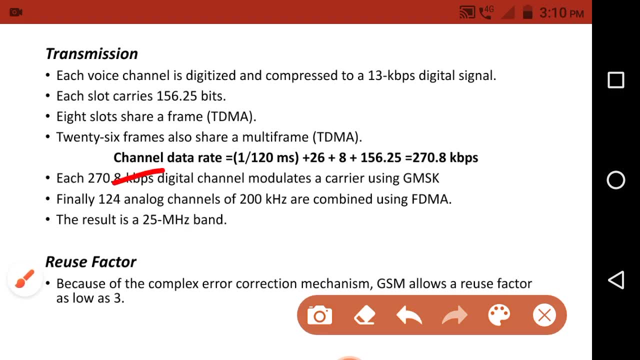 second. so how to calculate this particular bandwidth of the beat rate? so here channel data rate is equal to okay. so here one slot has contains the 156 point. two to five beats, okay, so there is a totally eight slots in the each frame, okay, and after like 26 frames are there. 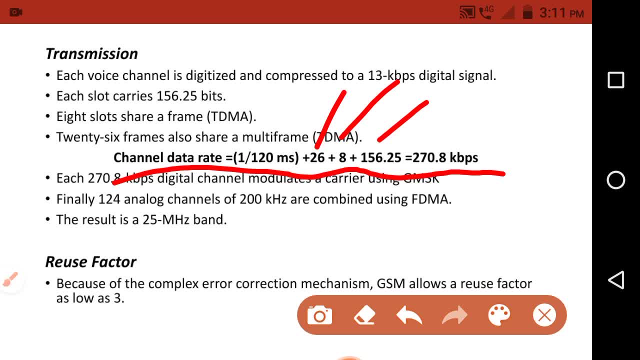 okay, totally, 26.25 frames are present. okay, and how much time we have to required? okay, how much time we have to required to send the one frame in the a multi frame, that is, a 1 by 120 millisecond. okay, so we need to make the addition of these all terms, then we will get the channel data. 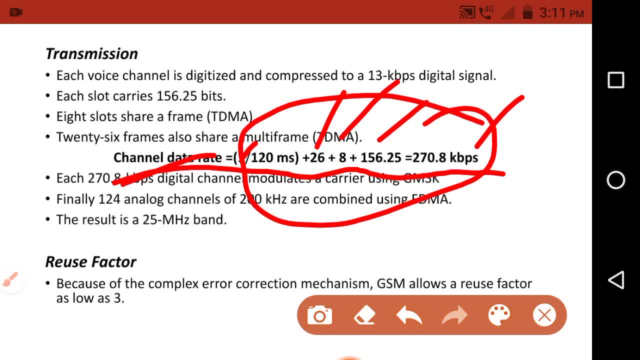 rate is 270.8 kilo b per second. okay, 156 is a beats we have to transmitted in the one slot. totally, eight slots are there? okay, eight slots will create the one frame. so here we are transmitting the 26 frame in one multi frame. okay, how much time we have to required to send the one multi. 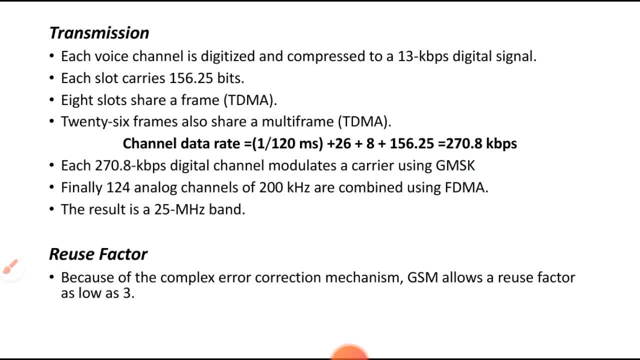 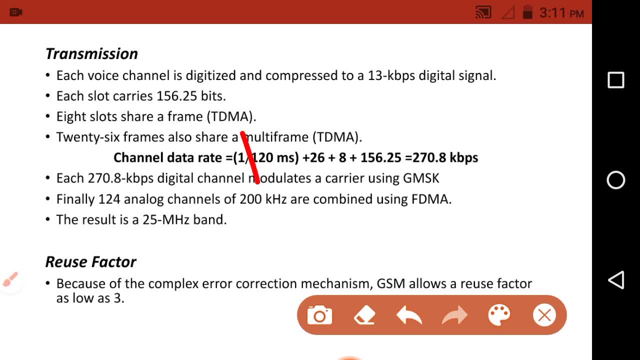 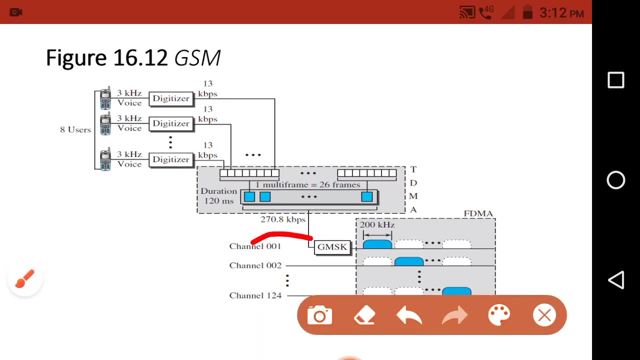 frame that is a 120 millisecond. okay, so here we need to take the how much time we have to required to send the one frame in the multi frame that is a 1 by 120 millisecond. oh, that will give the channel rate as a 270.8 Kobe per second. so in this way we have to calculate the bitrate: that is a 270.8. 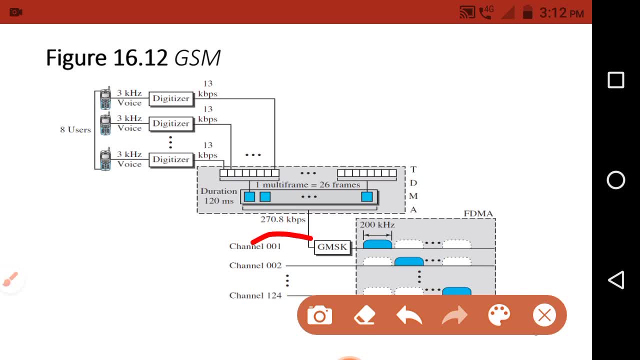 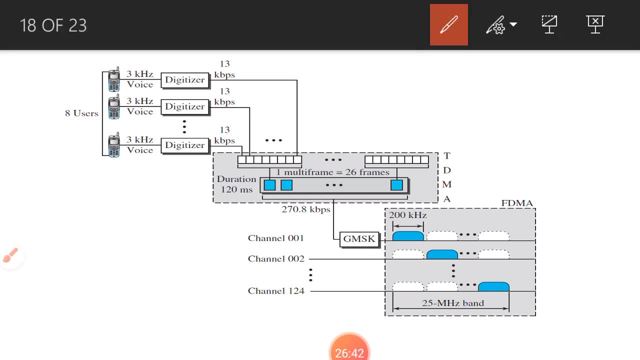 kilo beats per second. okay, so next, so next year űies 270.8 kilo beats per second. digital kicking 20 vezes per second. 0.own thousand, a sign we need to modulate into the analog signal, in the analog signal of 200. 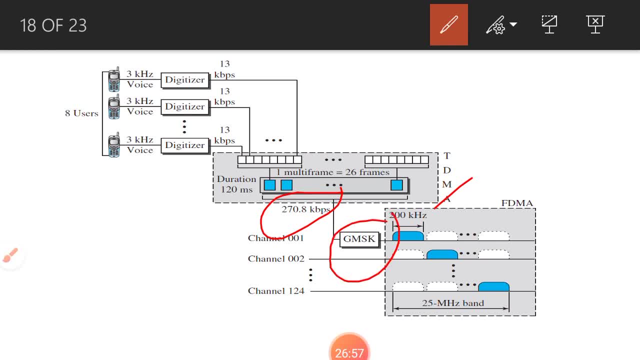 kilohertz by using the jmsk. jmsk is nothing but other. it is the one of the standard form of frequency shift key. it is a one of the standard form of the frequency shift key. so by using that standard form, we need to modulate the. 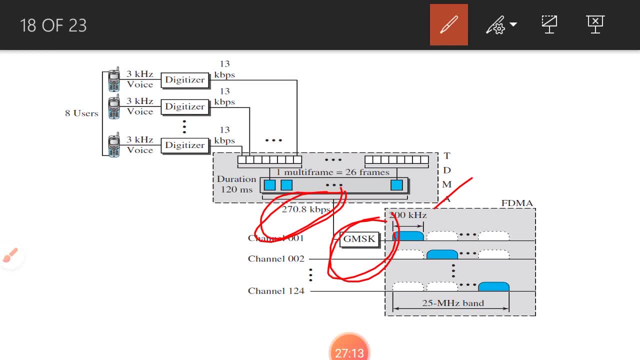 digital signal of 278 point kilo beat per second into the analog signal. there is a 200 kilohertz. okay, and here the 200 kilohertz signal will share the 25 megahertz bandwidth by using the FDMA, that is, a frequency division multiple. 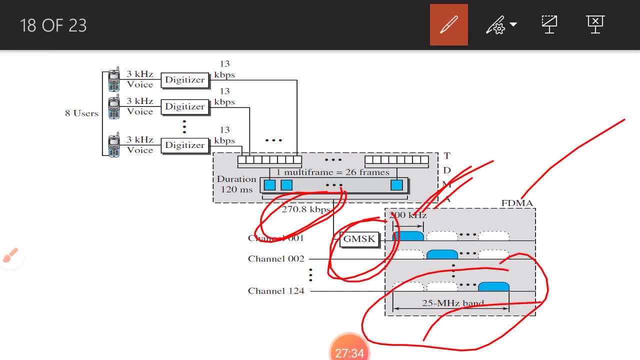 axis technique. so these 25 megahertz values, we have to divide it into the 124, as already we discussed here. so there is a 25 megahertz, so each forward and reverse band has contains a 25 megahertz bandwidth, so that each band has been divided into the 124 channel and 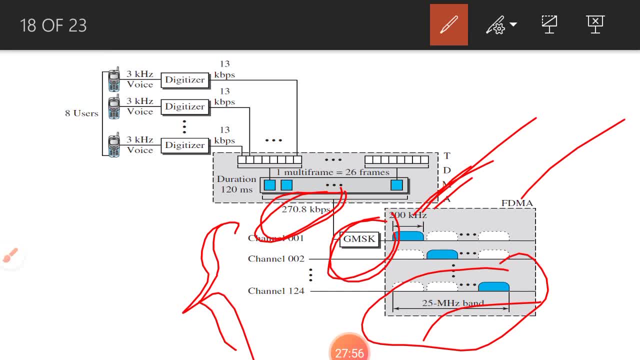 each channel has a 200 kilohertz bandwidth, so these 200 kilohertz bandwidth will share this 25 megahertz bandwidth by using the FDMA, that is, a frequency division. multiple axis means we need to allocate the fixed band, fixed frequency band, to the 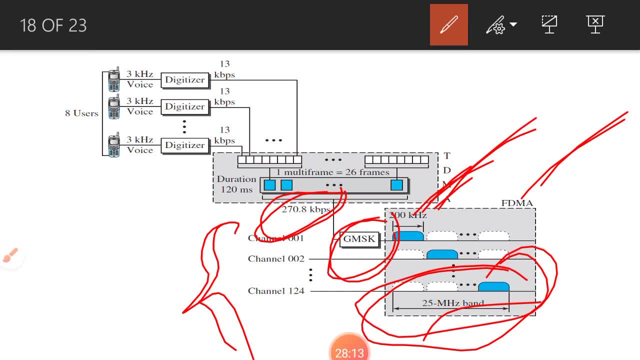 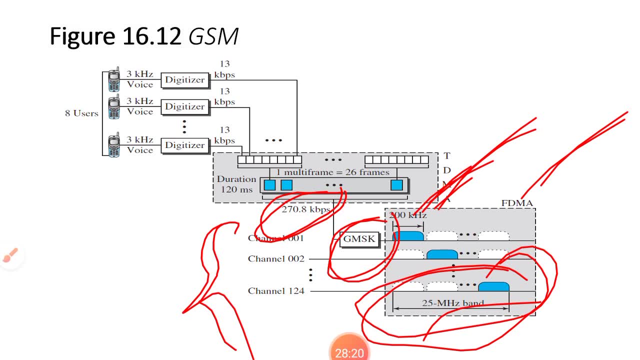 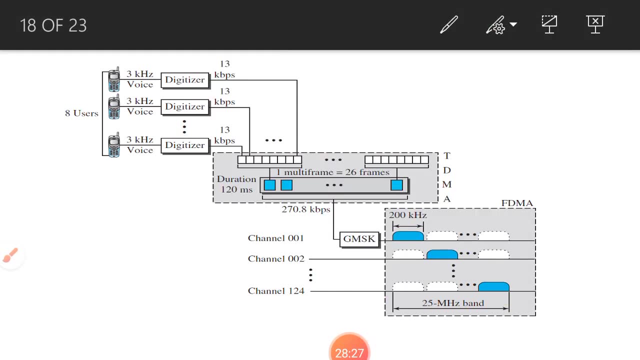 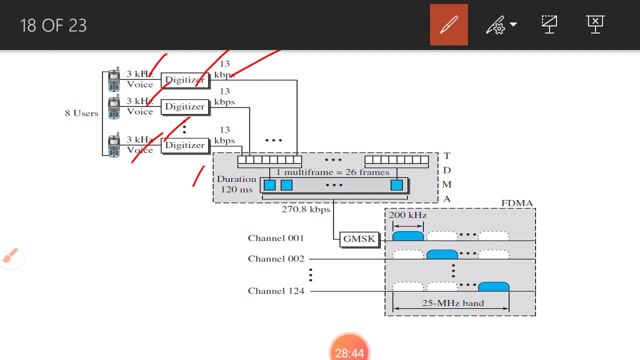 this is called the corral, that's analog wire signal into the disturbance. these are the variables for the 2x, and after that we need to combine how these frames are. the 8 bit frames are shared in the 1 multi frame by using the TDMA technique means here 1 multi frame is equal to the 26 frames. ok, and the duration required to send 1 multi frame is, that is, a 120 millisecond, ok. 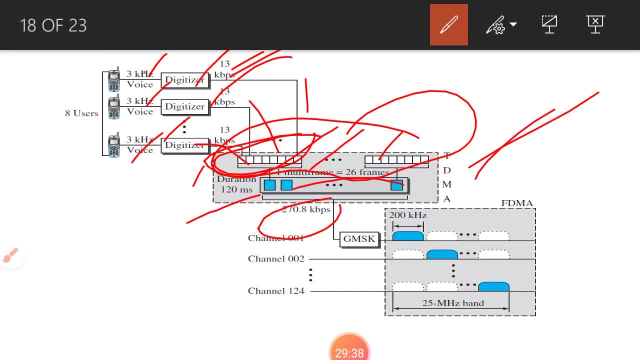 so the total bandwidth of the combined channel like channel which are combined through the TDMA technique is 270.8 KBit per second. and these digital signal we need to modulate by using the GMSK that is one of the standard form of the frequency shift K that will modulate digital signal into the 200 KHz analog signal that will share the 25 MHz bandwidth by using the frequency diffusion multiple axis. 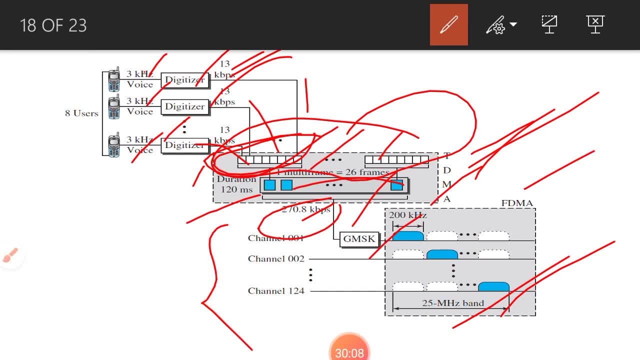 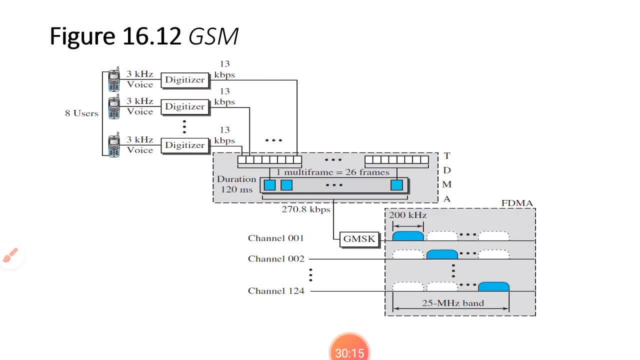 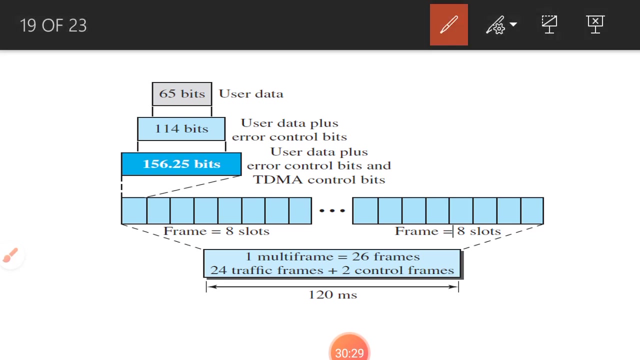 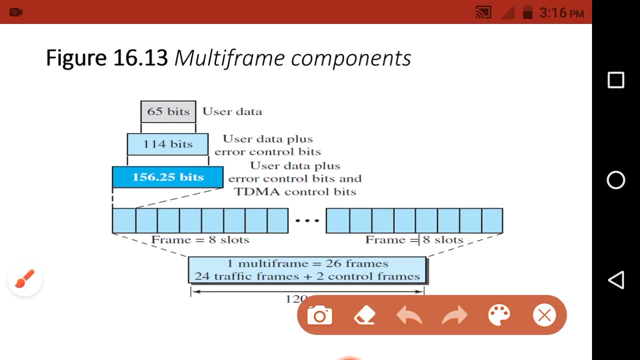 megahertz bandwidth, we have to divide it into the 124 channels. okay, so this is a what- GSM, global system for mobile communication. okay, and up to that, we discuss the what is a multi frame? multi frame components here. okay, so here what happen? multi frame components: we will discuss here. so here the each slot for: 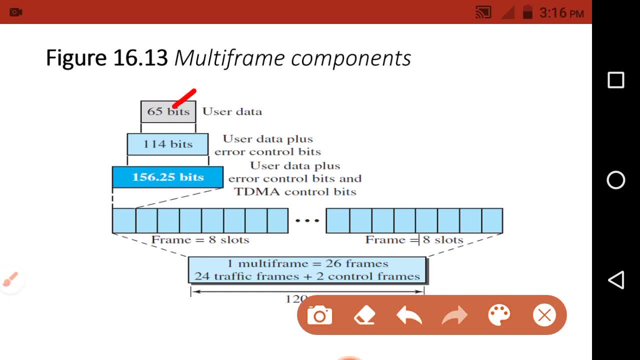 the each slot, we have to allocated 65 beats for the user data. okay, each slots of the frame: okay. so here, for the each slots of the frame, we have allocated 65 beats for the user data, okay. and for that user data, we need to add the some error control beats. okay, we need to add the some error control beats. 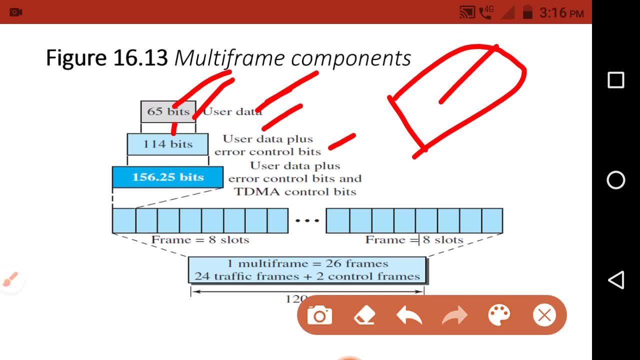 to that user data and that will be increases into the 114 beats per slot. and after that we need to add the some TDMA time division multiple access control beat to the error control beat and the user data and that will increase the beats to the 156.25 beats per. 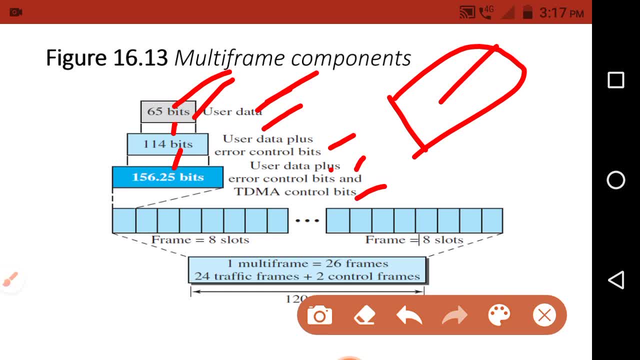 time slot. okay, so that is a nothing but one slot has contains the totally 156 point two, five beats, okay. such a eight slots will form the one frame. okay, and such a twenty six frames will form one, a multi frame. that is the one multi frame is. 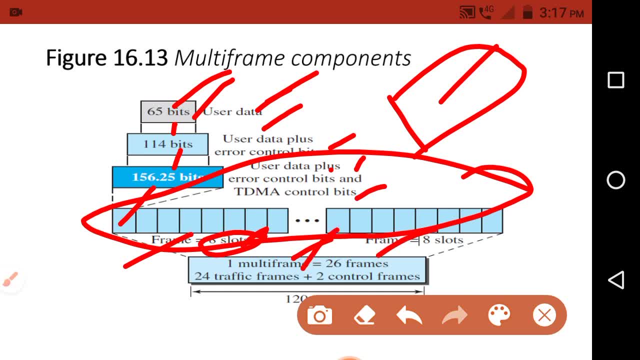 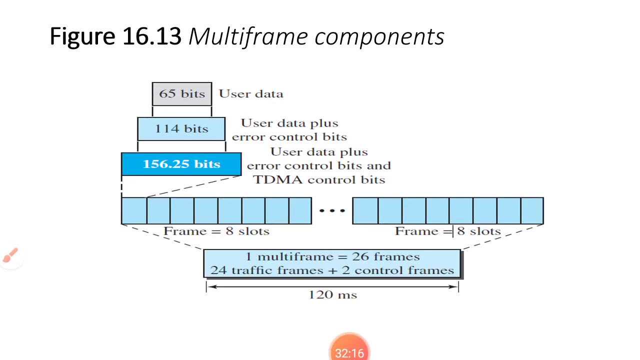 equal to the twenty six frames and each frame has a eight slots among those 26 six frame or twenty four frames we have to use for the wise communication or that traffic frames- okay, and two frames we have to use for him control the communication- okay, and total duration we have to required is 120 millisecond to 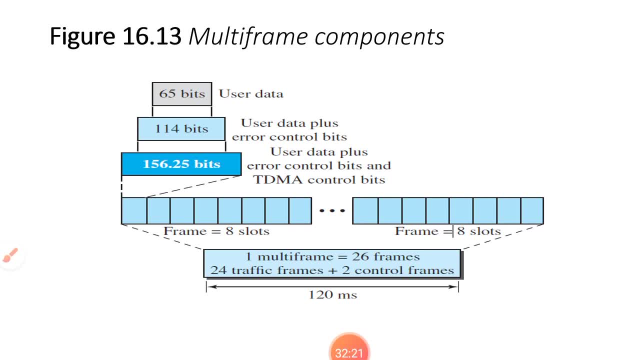 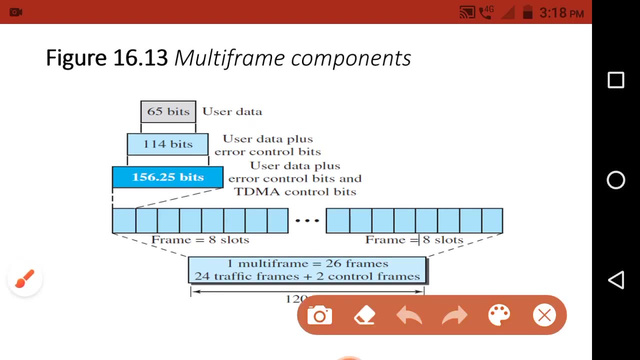 transmit the one multi frame over the channel. okay, so that's why they are given the 120 millisecond for the one multi frame. they are used for control the communication. okay, and total duration we have to required is one 20 ms to transmit multi frame. ok, so this is the multi frame component. ok, so 65 bits we have to allocate.